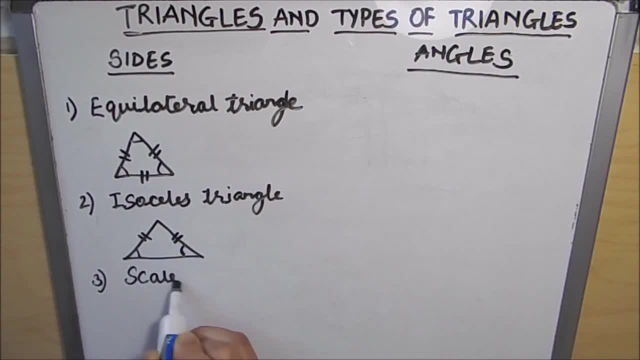 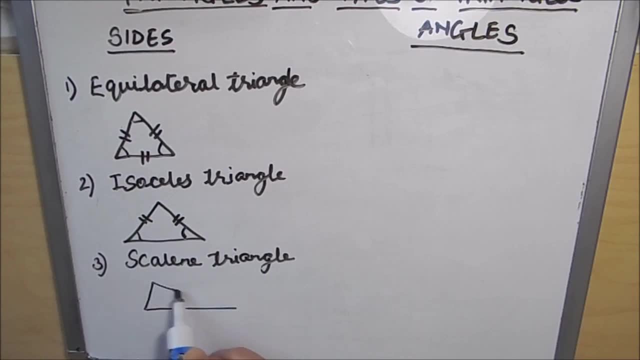 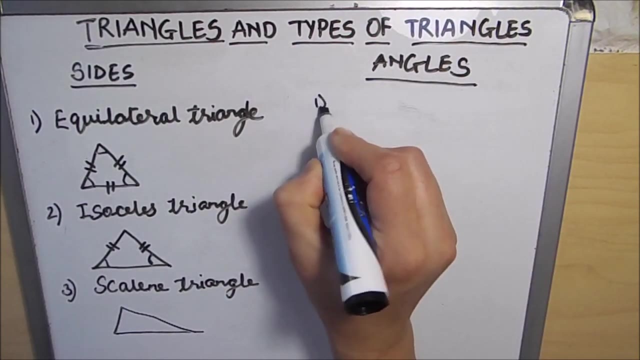 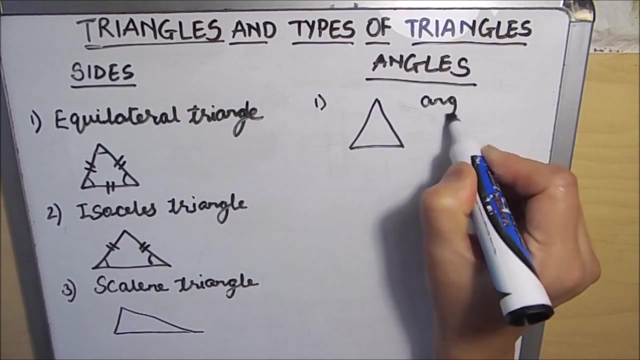 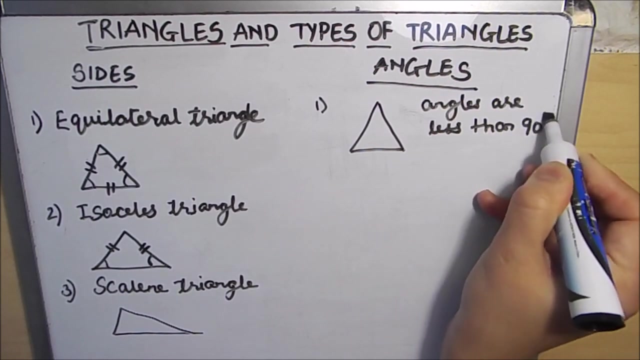 The third one is scalene triangle. So scalene triangle is a triangle in which all the sides are of different length. So triangles have also been classified according to their angles. So if all the angles of a triangle are less than 90 degrees, angles are less than 90 degrees called an acute angle triangle. 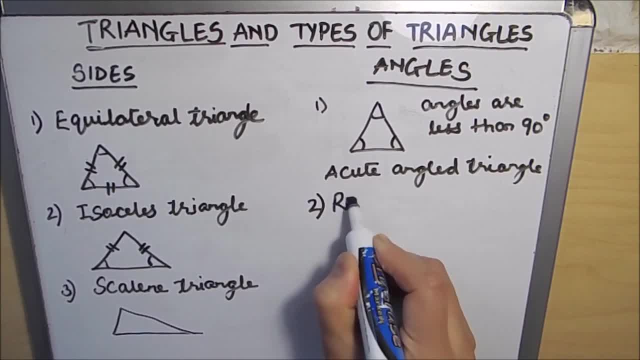 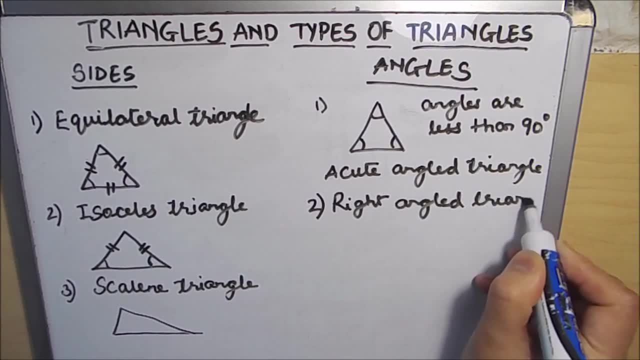 The second one is right angle triangle. So if any one of the angles of a triangle, if one angle is equal to 90 degrees, then it is called a right angled triangle. So here we see that one of the angle is 90 degrees, then it is called a right angled triangle. 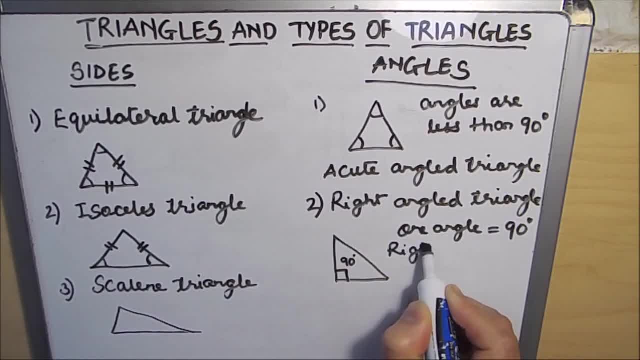 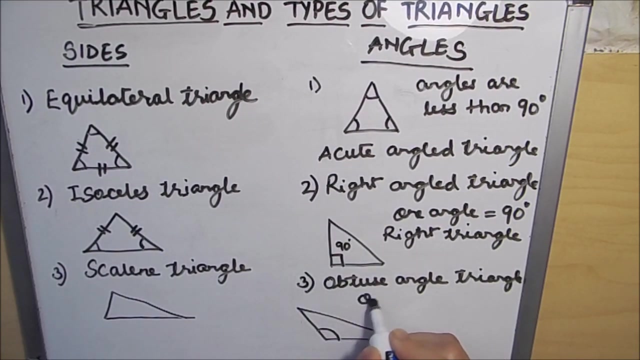 Right angled triangle is also called a right angled triangle. And the third category is the obtuse angle triangle. If only one of the angles of a triangle is greater than 90 degrees, then it is called an obtuse angle triangle. Right angled triangle is also called a right angled triangle. 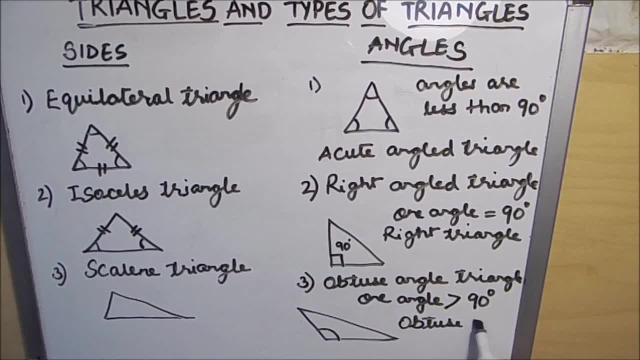 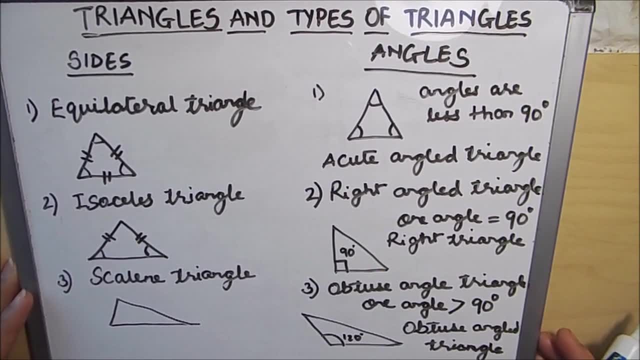 If only one of the angles of a triangle is greater than 90 degrees, then it is called an obtuse angle triangle. So here we have classified triangles according to their sides and according to their angles. According to the sides, we have classified triangles as equilateral triangle, in which all the sides are equal. 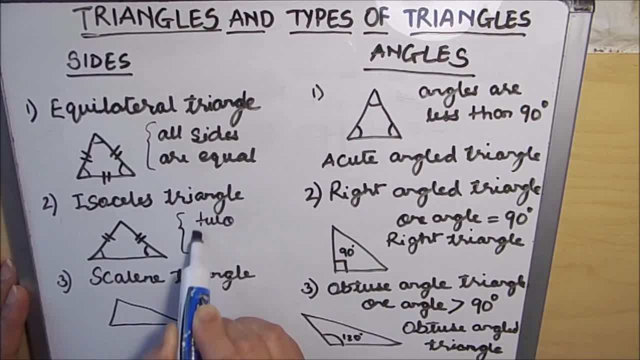 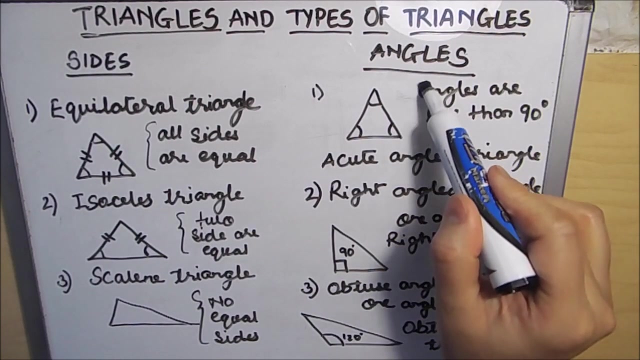 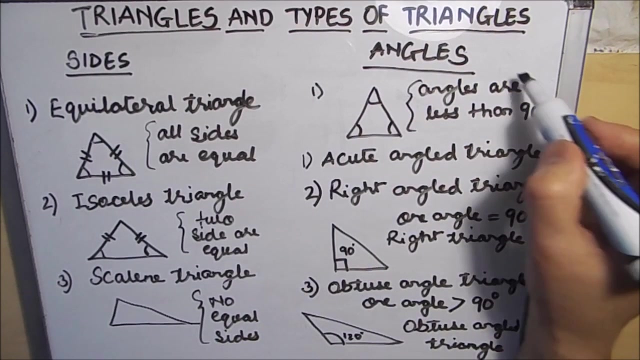 isosceles triangle in which two sides are equal. we have classified all the angles less than 90 degrees and scalene triangle in which no equal side is given anand scala tree angle in which there are no equal sides. These are according to the sides and according to the angles of a triangle. triangles are classified as acute angle triangle in which all the angles are less than 90 degrees.